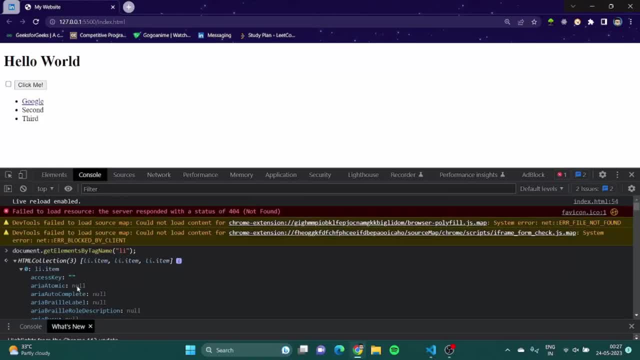 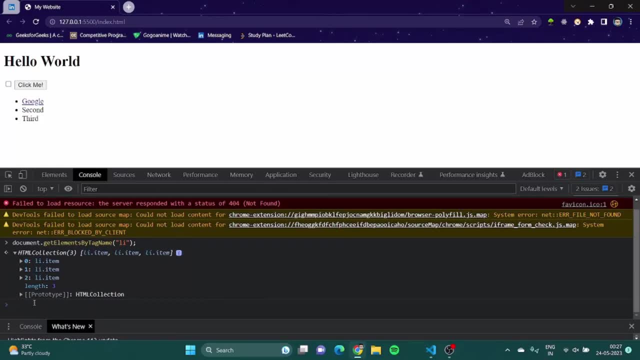 every item has different, different, different properties which you can tap and change. okay, great, now so you cannot um, like what we did in the previous video. you cannot change the color. okay, sorry, some spelling error: document dot. let's say: get element by. get elements by tag name. 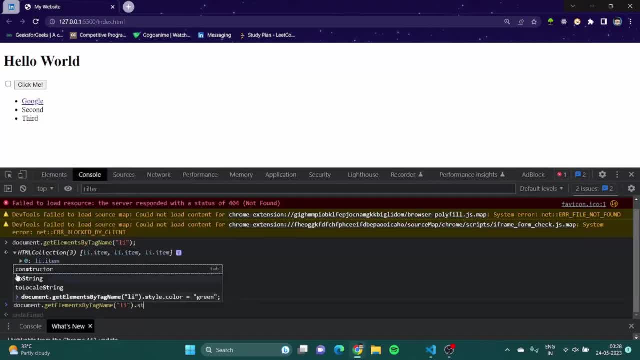 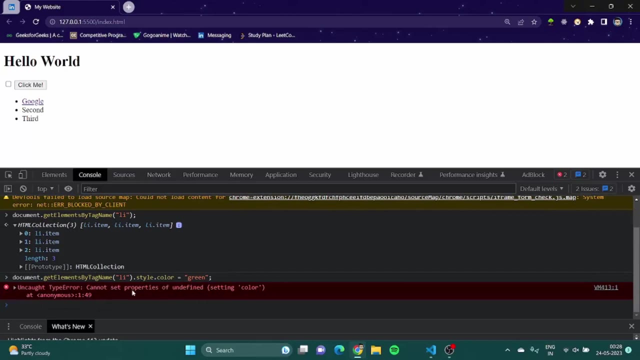 li dot style. let's try and change the color to green. okay, let's see what would happen. there's an error. cannot set properties. okay, the error is very vague, but let me tell you what the error is. so document dot get element by tag name. li basically selects this whole array. okay, of three. 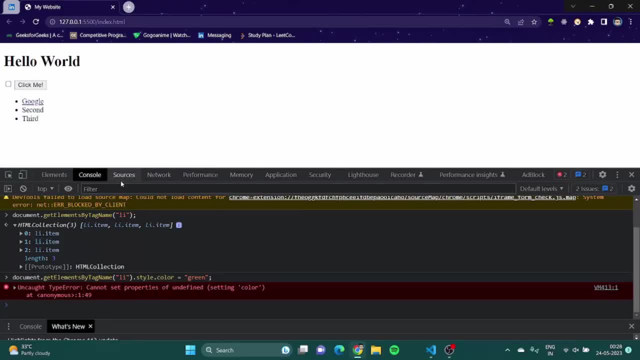 items, which are google, second and third. okay, then we're going to set the respective elements to this. this is a link. uh, now, obviously you cannot change the color of an array, so what to do in this case? let me just copy this whole thing, i'll just paste it and here, like array, you can tap in any element. 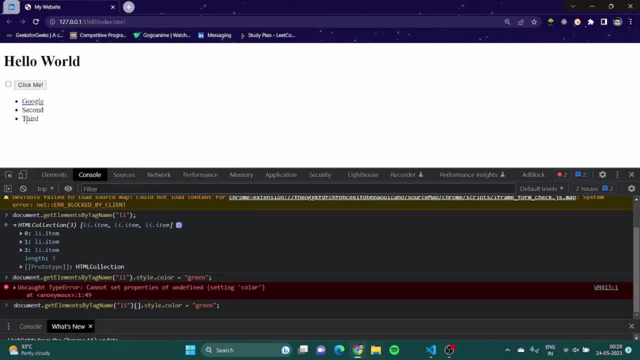 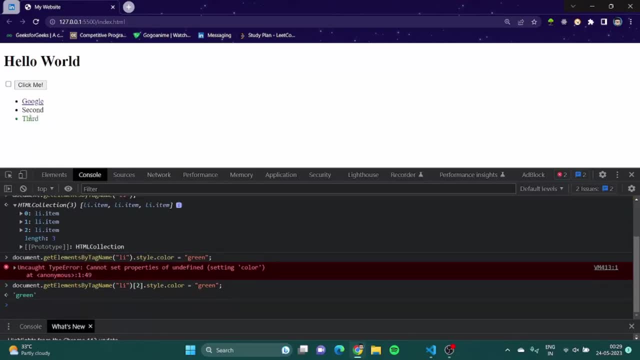 of array using a square bracket. let's say you want to change the color of third, so we'll just say two and yeah, you can see it has turned to green. okay, now i hope you remember how arrays work and how to tap in elements of an array. if you don't, i have made a video over arrays where i have taught. 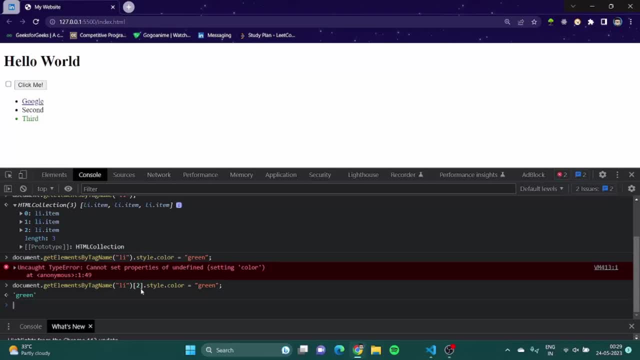 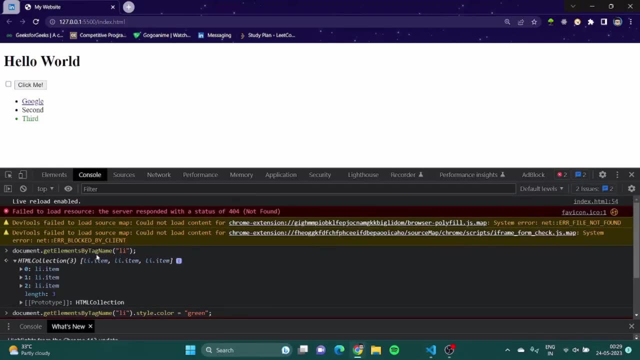 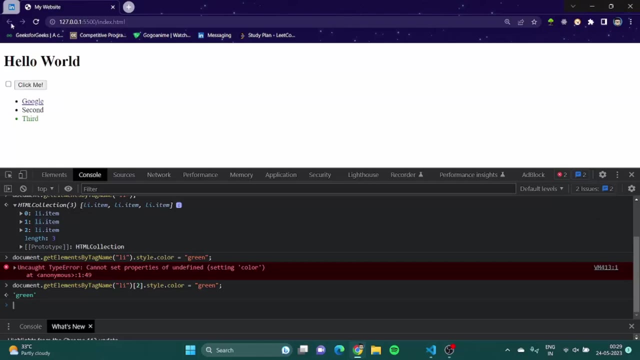 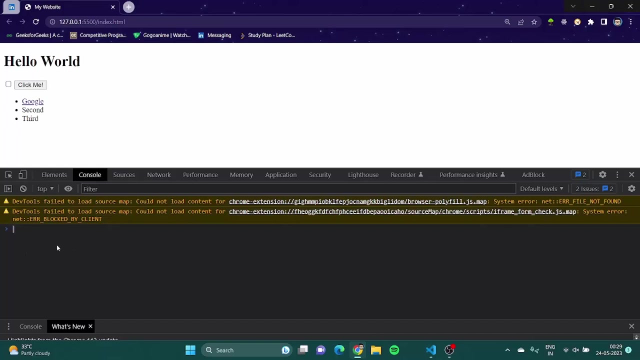 it in detail so you may check out that link. okay, great, now this was all we had to talk about tag names. okay, now, what we can do. what we can do. what we can do is we can just refresh the page, get it fresh. now there is another thing called class name. get elements by class name. so what you can do, 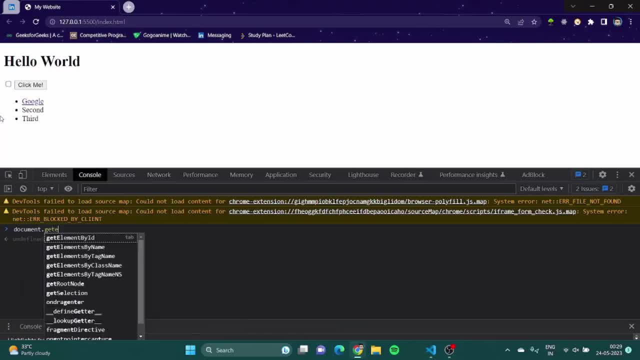 you can simply go document, dot, get elements by class name and here you can give it any class. let's say: uh, button of class btn, uh, btn, okay, great, it has returned me. uh, again, see, it is element. so again it would return me. what an array, right. so again, uh, if you want, you cannot simply do what uh, dot style, dot color. 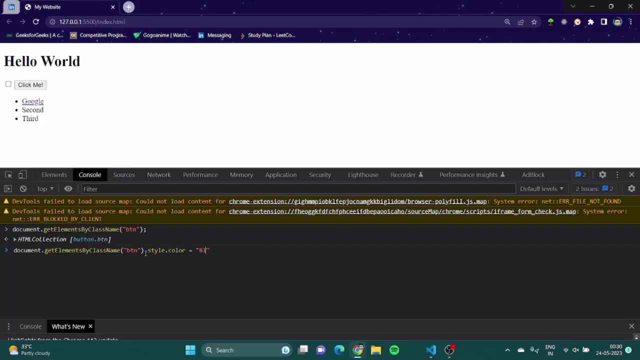 is equal to, let's say, blue. it cannot do that because, again, it is what single element? i mean an array. so to tap in the element, you can simply do this and see it has turned to blue. okay, great, that is what i was talking about and that is how it works. okay, now you can. 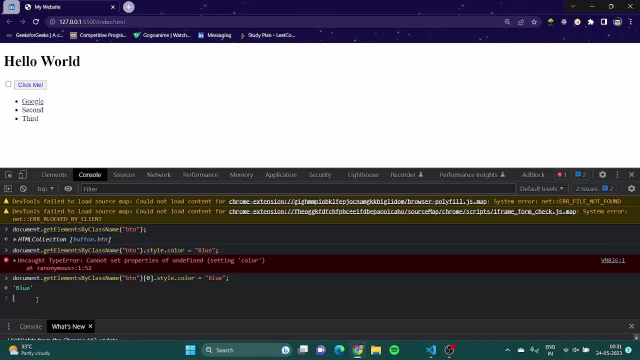 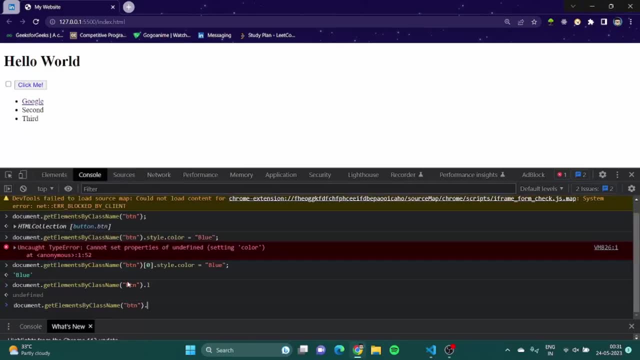 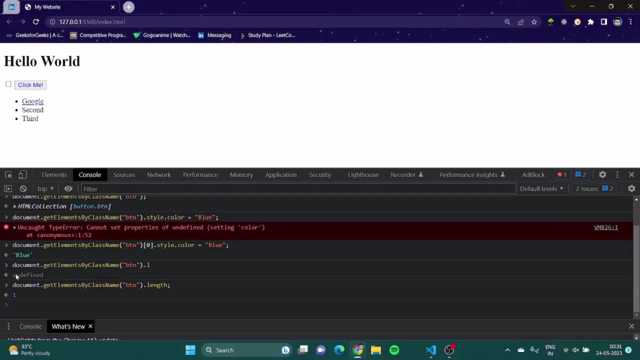 do one thing. if i just copy this, you can see other properties of arrays. like you can simply write: okay, dot, let's say length one, because single element. okay, so you can see this document. this selects the items with the class name buttons and gives you view, a list and then, um, like arre list that you know how to change it. i mean how to 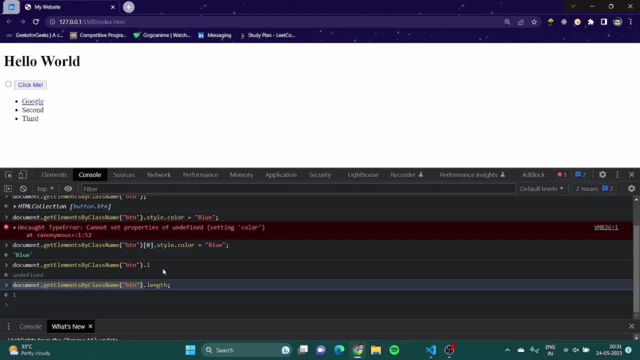 work with it. you can, you know, find it and use it or display it, but you can also use it by this method: its length, find any particular element, do something over it, etc. okay, that is up to you all, right, great, that is what i wanted to talk to you about. uh, in this um elements by class name. 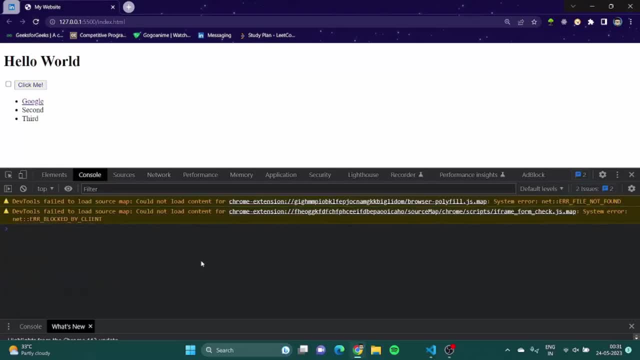 okay, great, again, i'll refresh it. and there is another method that can be used to select a single element. okay, i think i gave you a lot about it, so rather than doing it, let's see again. you will say document, dot, get, and the key ones might have noticed that here it is only an element, not elements. again, it is. 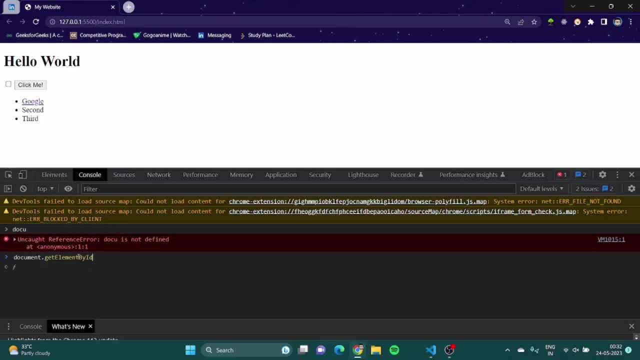 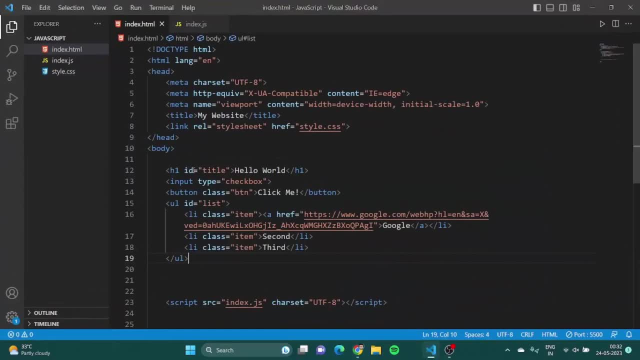 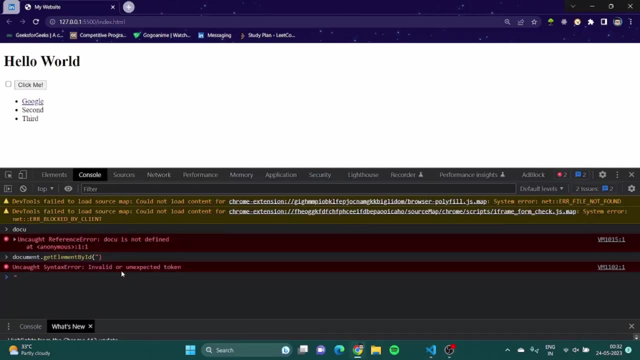 very obvious, because on a single web page there has to be unique id, so obviously it would return me only a single element. if i check, it is ideas title. let's see if i write okay, what the hell happened. sorry, let me just refresh it so we can start from fresh. yeah, 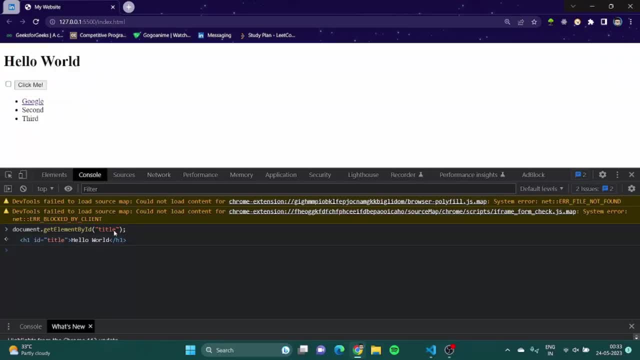 see, it has written me a single element with h1 id title. now i can change it in a i mean text by saying inner html to: let's say good bye. see, it has changed. so that is how let's get element by id works. okay, now another method that can be used to select a single element is 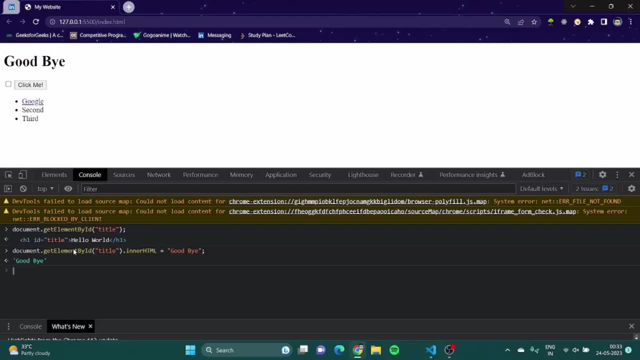 is the query selector method that we have used in the previous lesson as well. now this method is, you know, similar to get element by id and it returns a single element, but it works a little bit differently because, okay, give me one second, let me type it out. so 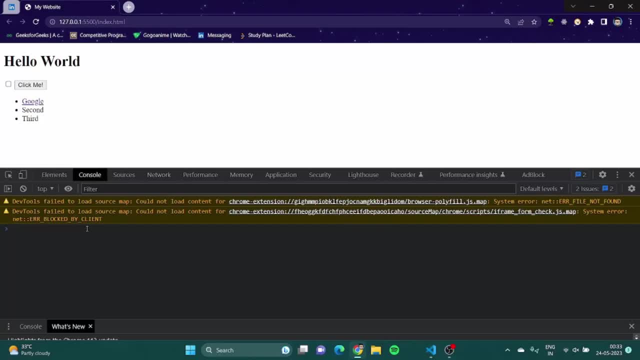 so, like it would be easy for you as well to see document. uh, okay, my hand dot query selector. okay, yeah, okay, okay, okay, great, great, great. all right now, whatever the text i want to write inside it, the string that you're going to put inside it, parentheses, is a selector. 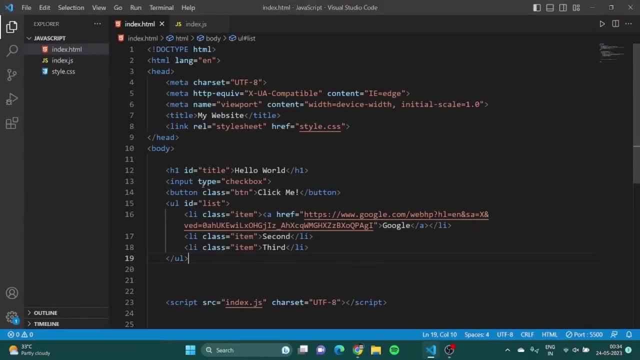 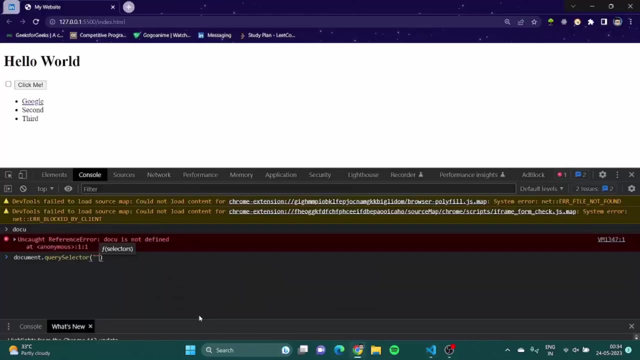 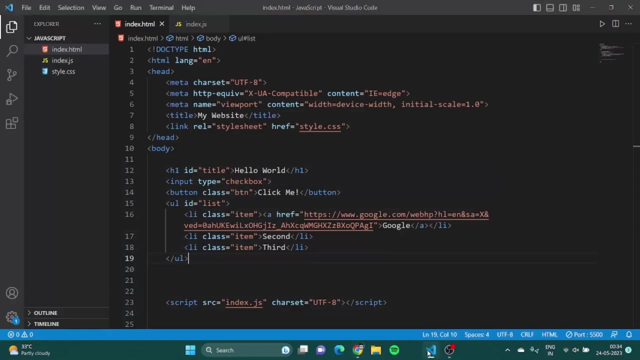 now, what is the selector? we have been using selector for all this. while id is a selector, class is a selector, this tag element is a selector. remember, whichever we use in css, that is a selector. so suppose if it is an id, so for that you have to use hash? uh, let's say id was, let's say title.